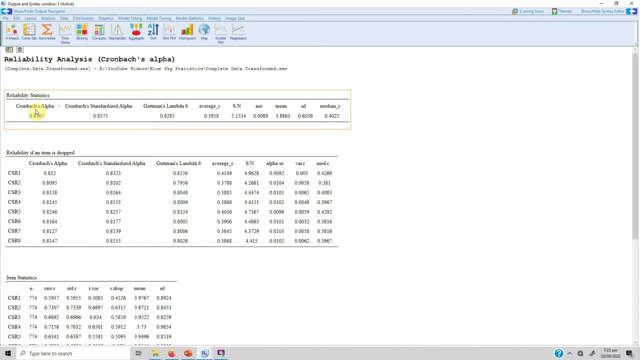 over 0.7.. So this means good reliability. If it's over 0.8, it's very good. If it's over 0.9, it's excellent. If it's greater than 0.6, it's fair. But if it's less than 0.6, there might 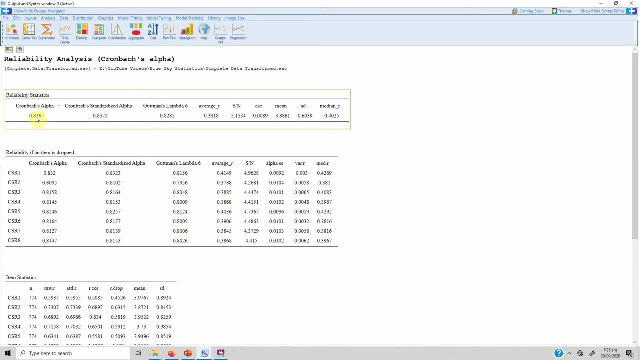 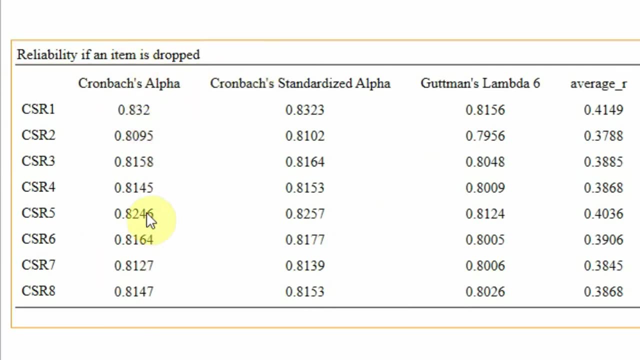 be something that you should be concerned with. And then what you do is you look into reliability if an item is dropped. So, for example, in this case, if we cannot drop any of the items because the reliability would not improve, Even if we would have improved reliability, 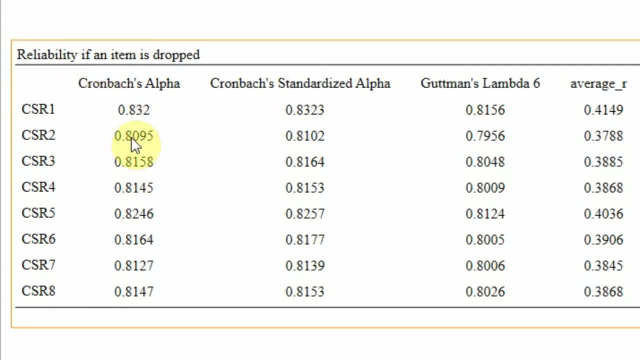 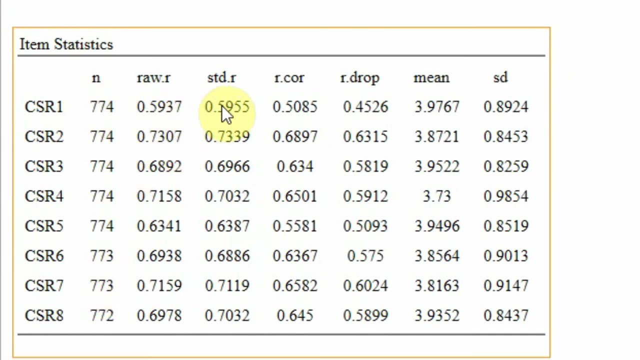 by removing an item. we have to see that how much the reliability is improved. If it's already very good, you do not need to delete item just to add a few decimal points to your reliability. In this case we are not going to delete any of the items. And here are your item statistics: The mean. 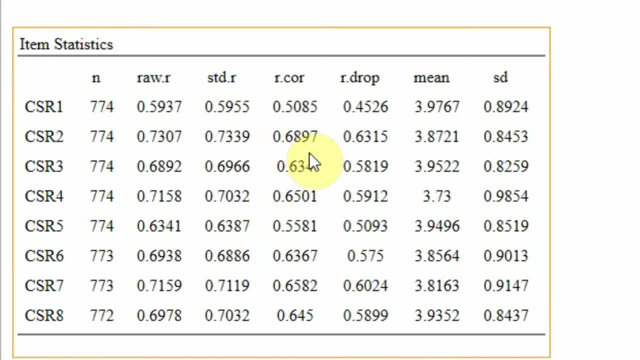 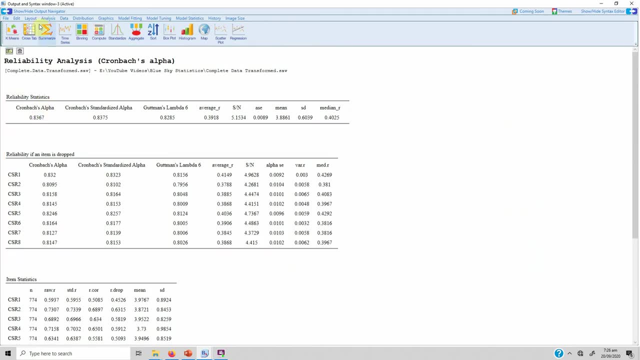 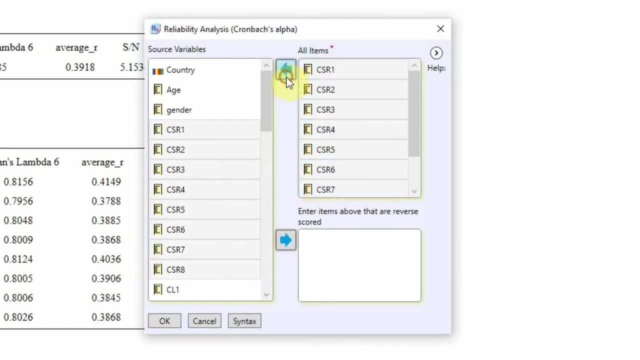 the standard deviation and the R correlation item to total correlation. it should be greater than 0.30. And in this case it's fine. Now let's say, let's do it for another one: Analysis, reliability, analysis. Let's remove all these from here. 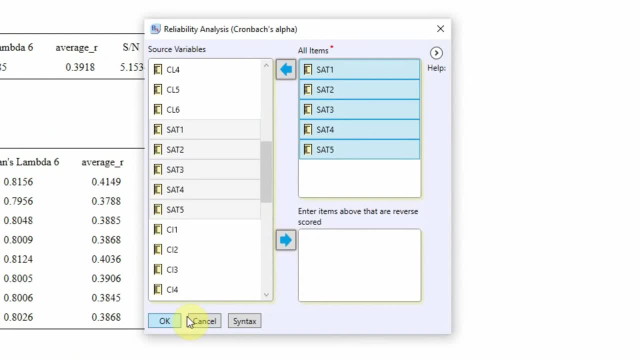 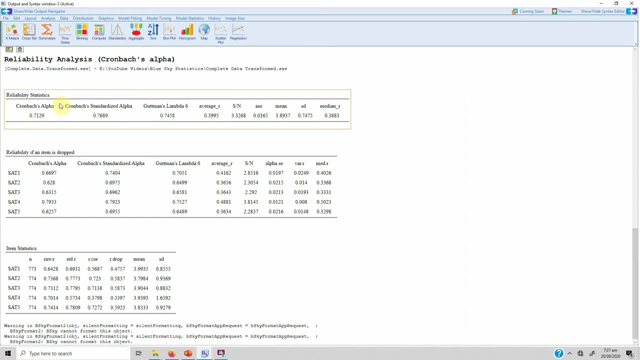 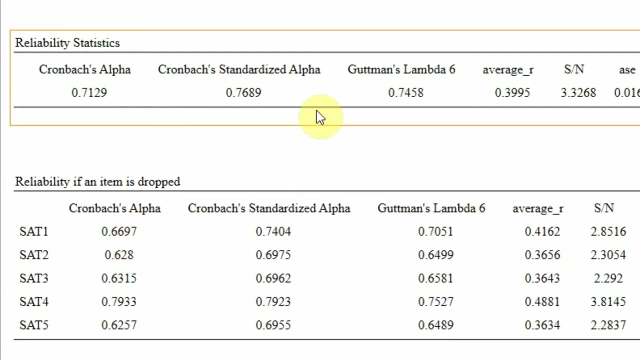 Let's do satisfaction. Put it in here. There are no reverse items. It's okay. And here are your results. The overall alpha value is 0.7129.. Now it's actually good because it's over 0.71.. If you remove satisfaction one, the reliability would decrease. If you remove. 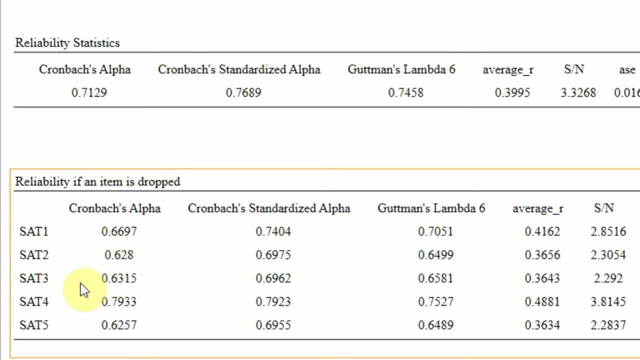 satisfaction two: the reliability would decrease. Remove the reliability would decrease. But look in here. Satisfaction four: If you remove this item, the reliability will actually improve And it will improve significantly from 0.71 to actually 0.79.. Now, what is the reason for this? If you look here: 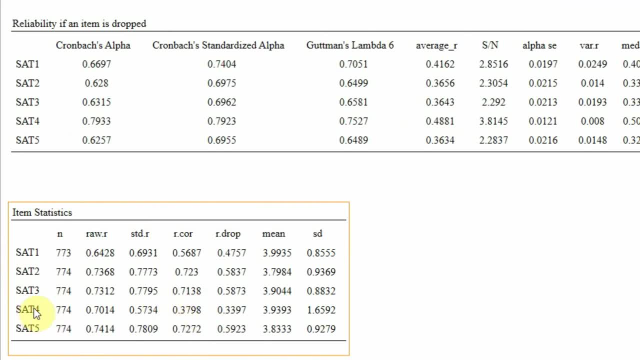 satisfaction. four: item to total correlation. the correlation of this particular item with the overall scale is 0.37,, which is actually low, Although it's higher than 0.30, but it is low. So you might consider removing this item, but in my experience I wouldn't do it because your overall 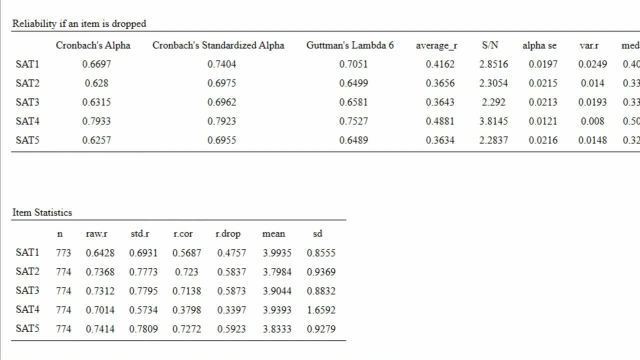 reliability is actually good, But what if it was less than 0.7?? What if it was 0.6129 rather than 0.7129?? So I will come down to this table And, if I look at this table, removing satisfaction four actually. 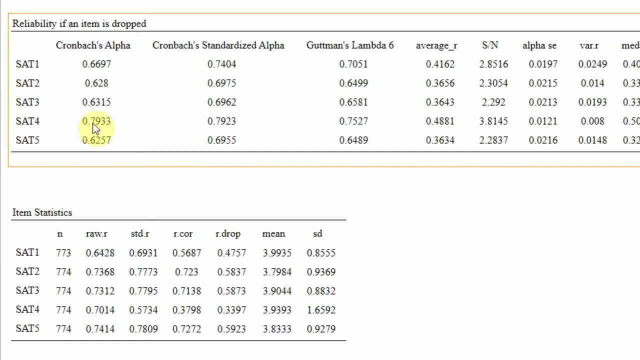 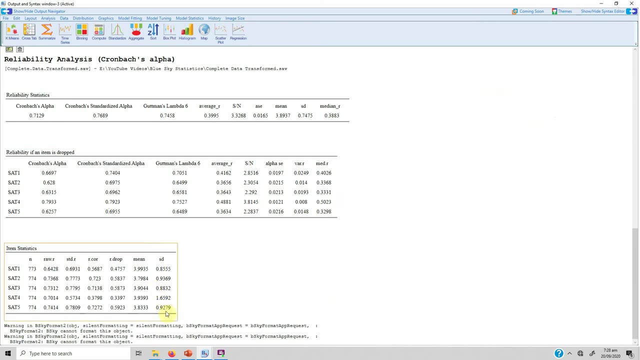 increases my reliability to 0.7933.. So, yes, I will delete this item And then improve my reliability. So this is how you can do reliability statistics in BlueSky Statistics. Now, how do you report reliability analysis? It's pretty plain and simple. Let's do this. Let's open. 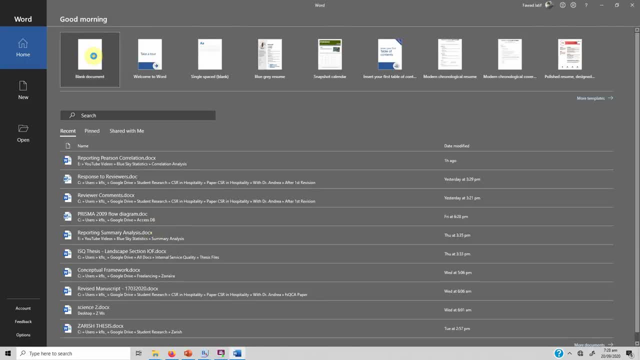 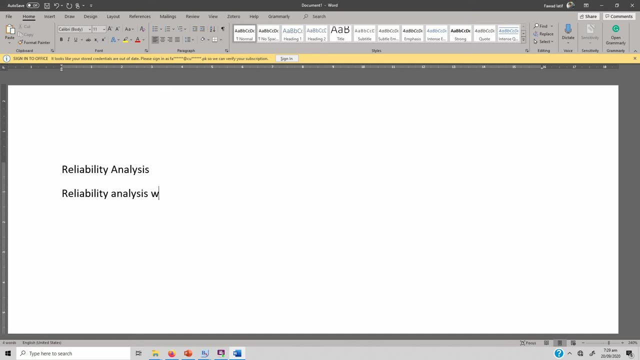 Microsoft Word And let's say we give a heading: reliability analysis. Reliability analysis was assessed using ground, That is, alpha. The results of reliability analysis revealed acceptable reliability for each of the constructs in the study. results are summarized in table 1 so you can put in. 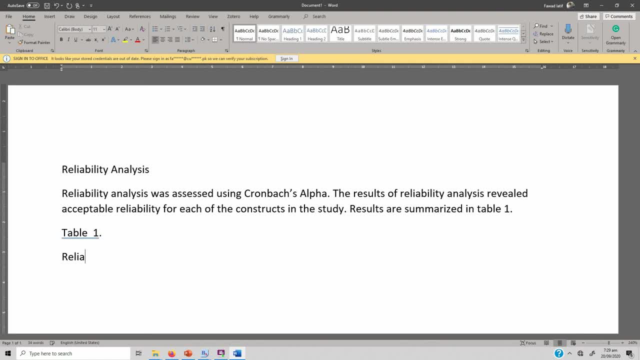 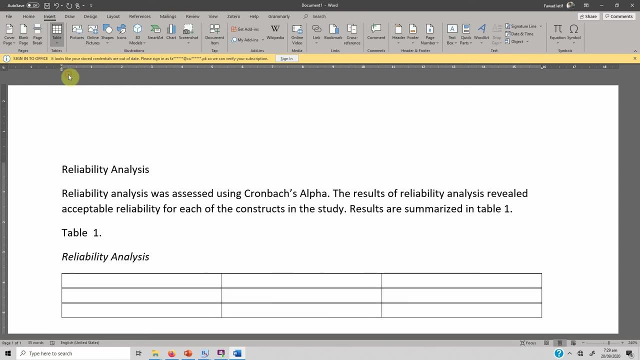 your table 1 here, ability analysis, italics. now add a table. this is for construct number of items from that alpha and let's say construct number of items, alpha value. that's it for CSR. it was satisfaction. number of items: 8, in this case 5, it was 0.87. 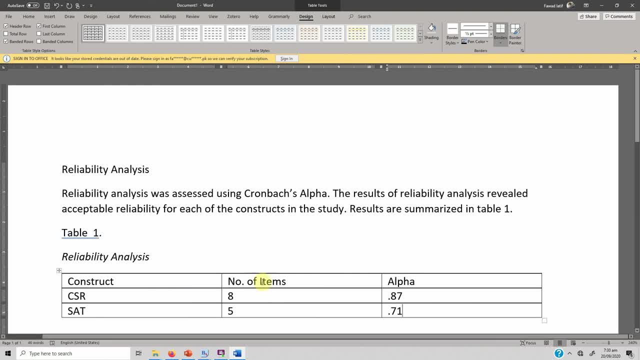 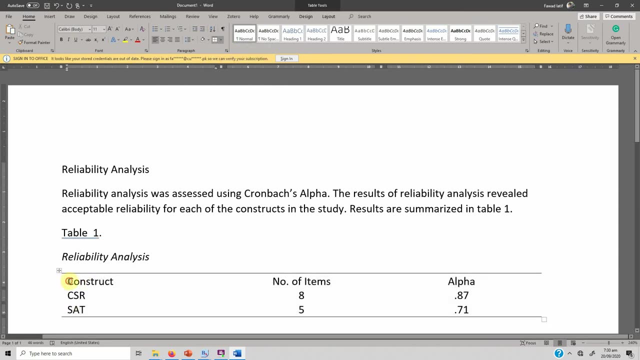 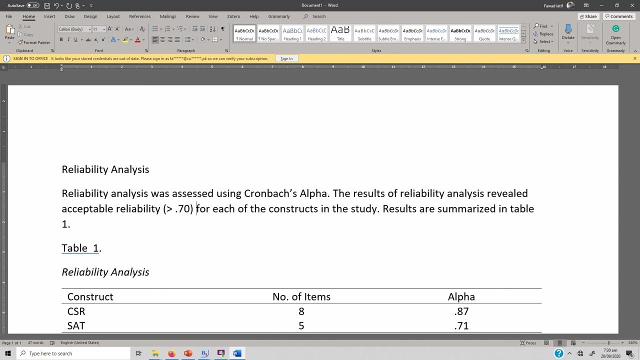 let's say, and it was 0.71. so this is how you can report your reliability analysis and let's like format it a bit. it's always a good idea to put in the acceptable reliability 0.70. it's greater than 0.70 for each of the construct and you can put in a reference as well here.